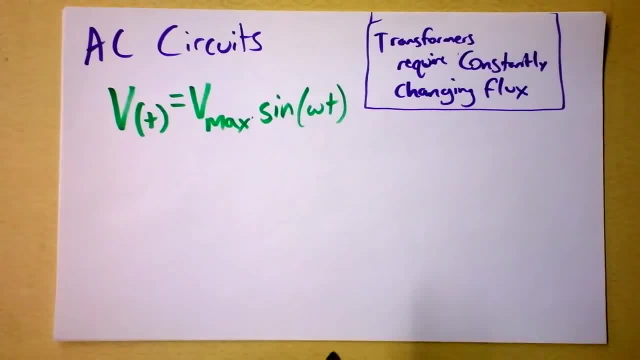 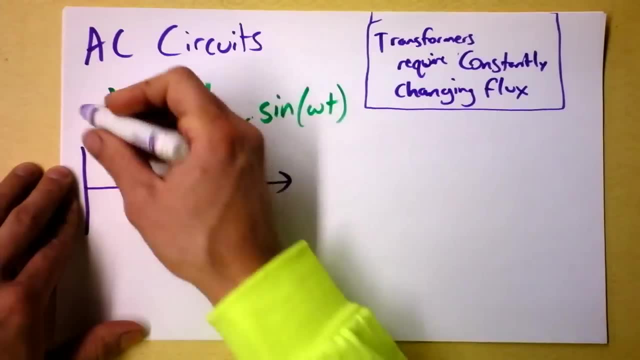 That's going to be in radians per second, So be careful. We're going to be taking the sine of something in radians And that gives us a graph of. let me get you the Vmax. This is voltage And this is time. 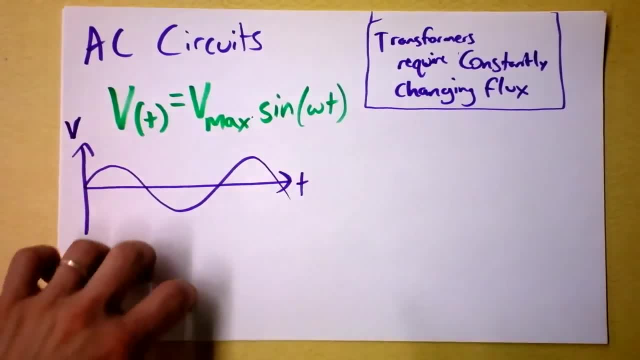 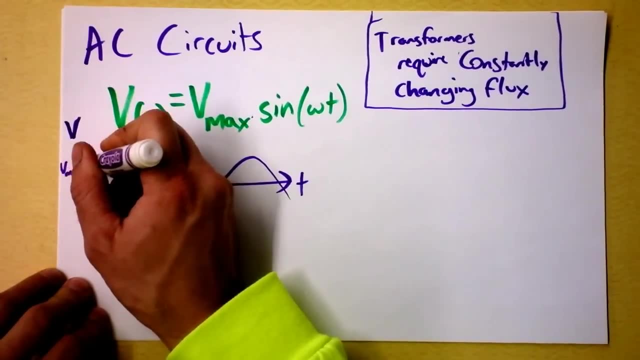 And it's going to start out here and go like that. So if the voltage is doing that, then this level right here would be Vmax. If the voltage is doing that and you've just got a simple resistor like I don't know, 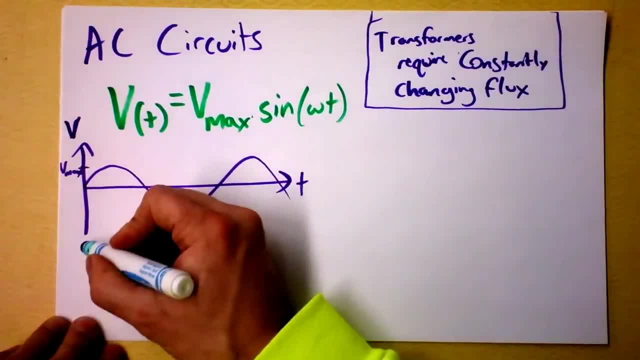 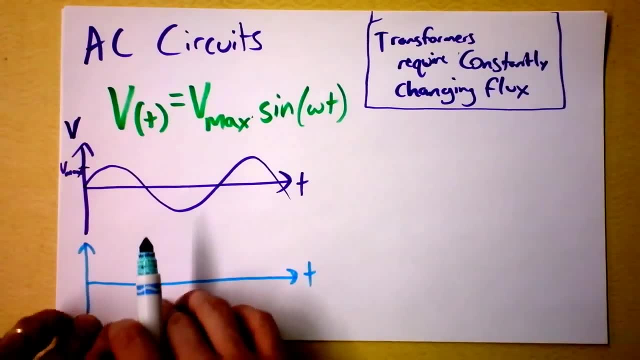 a hot plate or a toaster or something, then the current will be doing, in fact, exactly the same thing. The current will be changing as a function of time. This is how hard you're pushing And this is the way the system responds. 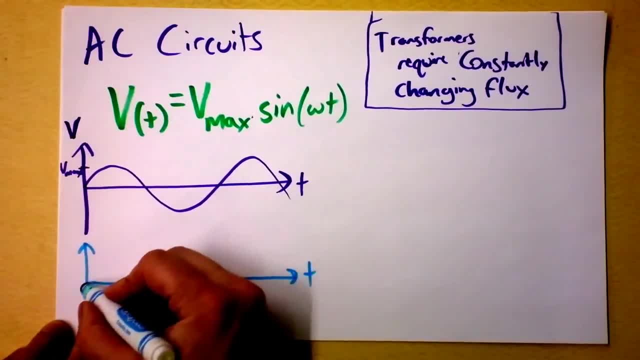 So it's kind of like a stress-strain relationship. Okay, So you're going to have the same relationship again And you're going to have- well, certainly you won't have the same value, But we'll expect the zeros to line up. 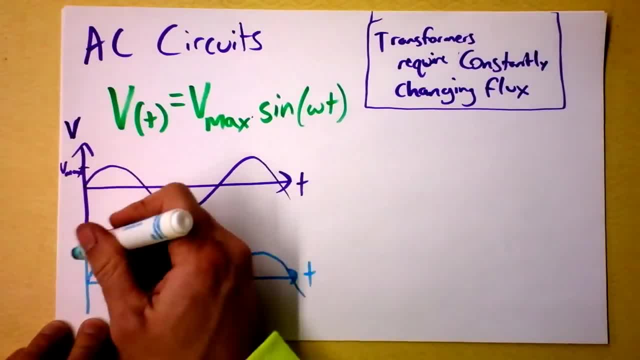 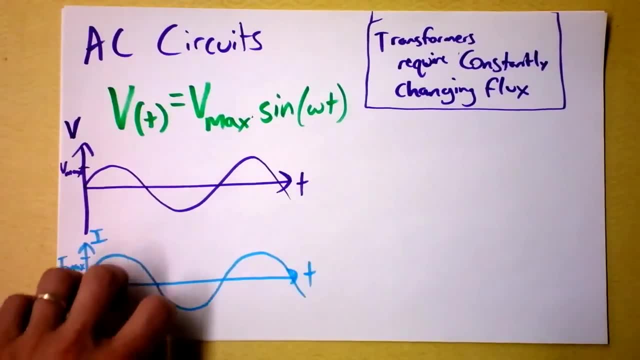 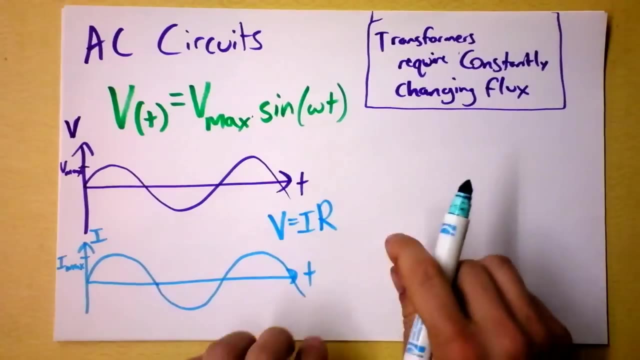 And we'll expect it to have the same structural performance here. This is current as a function of time, And this is Imax right here, And we've still got all of our favorite relationships like V is IR, But all of these become a function of time. 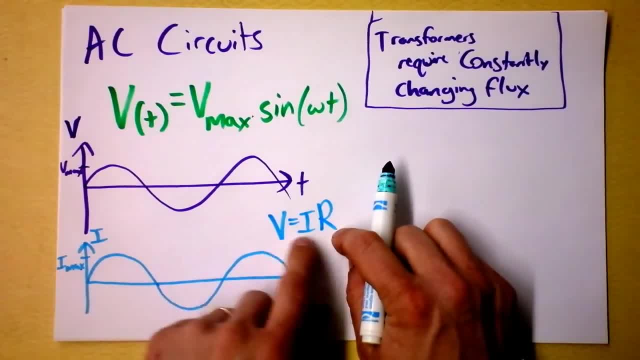 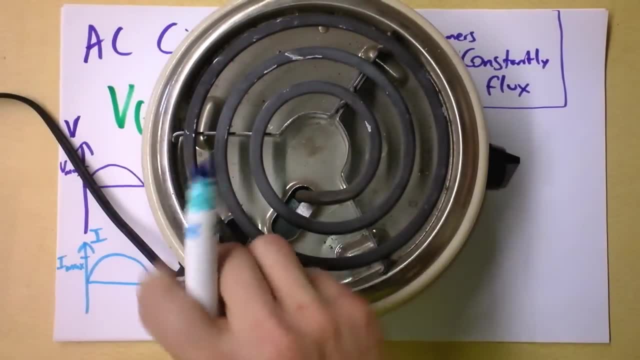 You assume that the resistance doesn't change with time, But if the voltage is going up and down And the current is similarly going up and down, So inside of my hot plate I actually have current going this direction and then that direction and this direction and that direction, clockwise and counterclockwise. 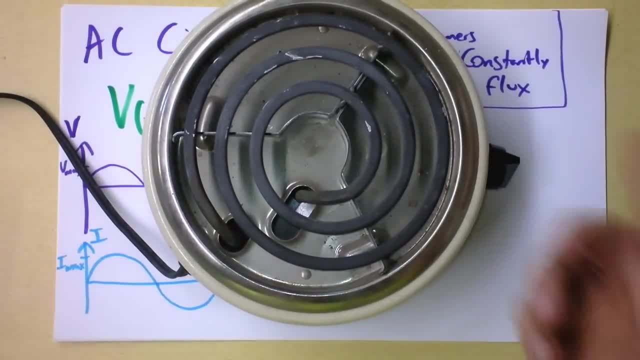 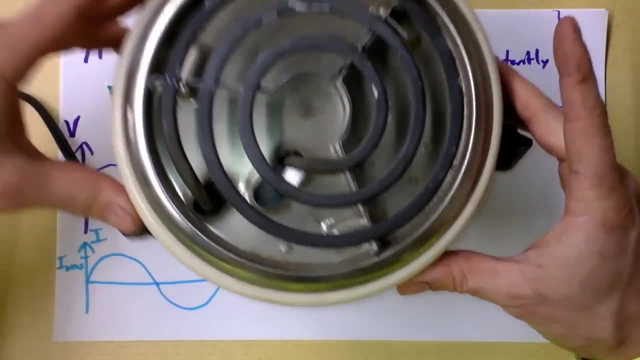 And in the United States it changes 60 times every second. It's going forward and back 60 times in every single second. And in Europe and India- shout out to India- I think they've got 50 times every second that it switches direction. 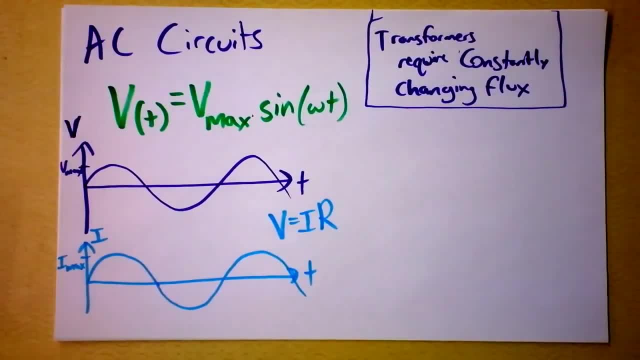 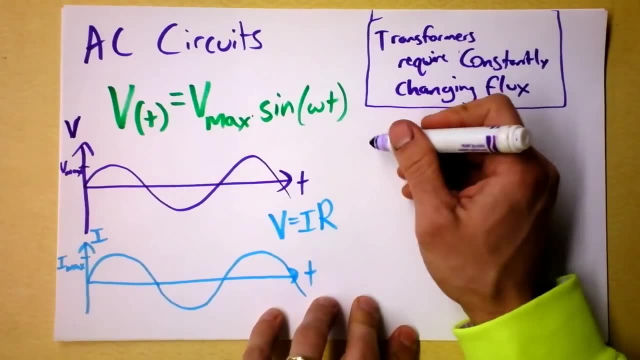 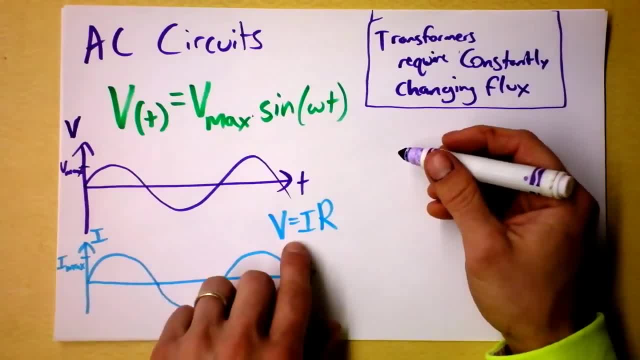 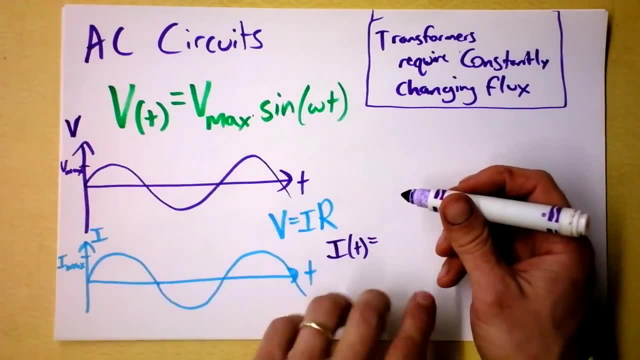 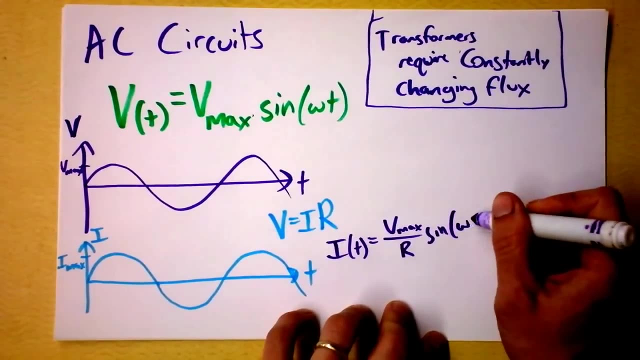 No, let's not try to find out what Vmax is. Let's just say that current as a function of time is going to be. well, I guess it'll be V as a function of time divided by R. So it's Vmax over R times the same sine function. 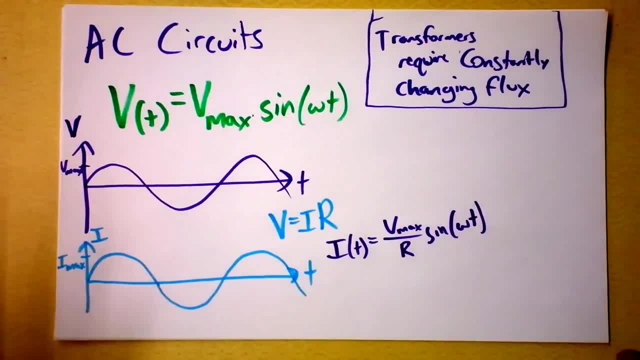 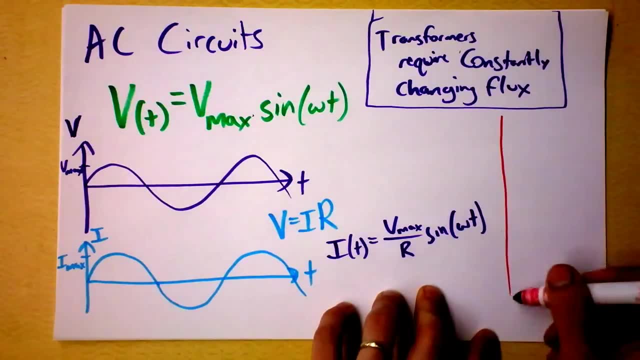 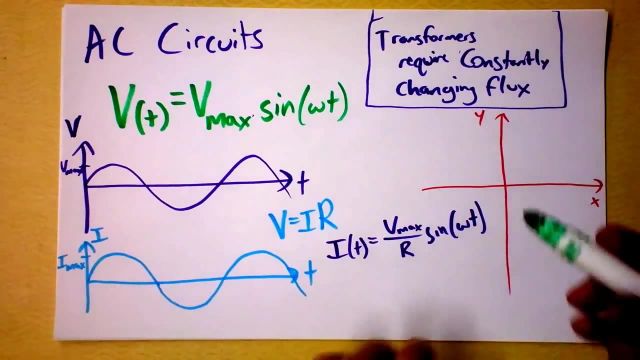 sine of omega times T. And now it's time to introduce a really neat concept. These things are called phasors, And a phasor looks like this: First you get yourself a coordinate system- And I'm just going to define x here and y here- And a phasor is a vector. A phasor, simply put, is just a vector. 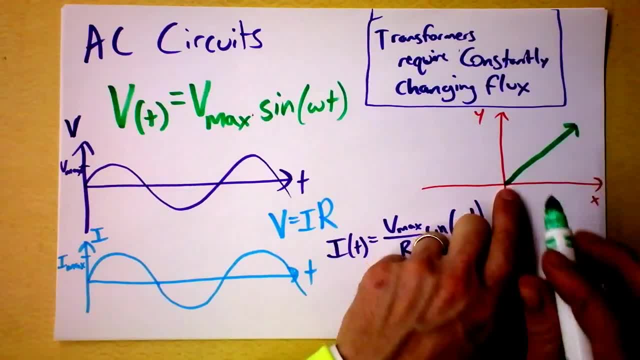 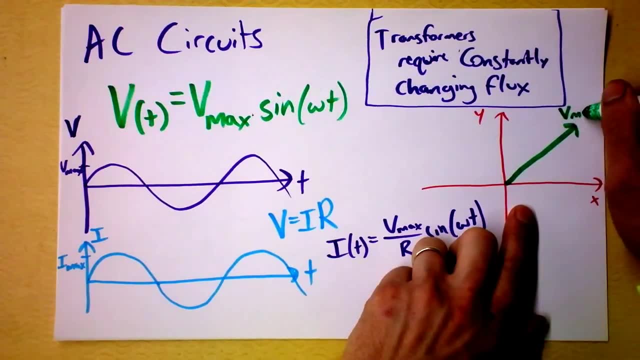 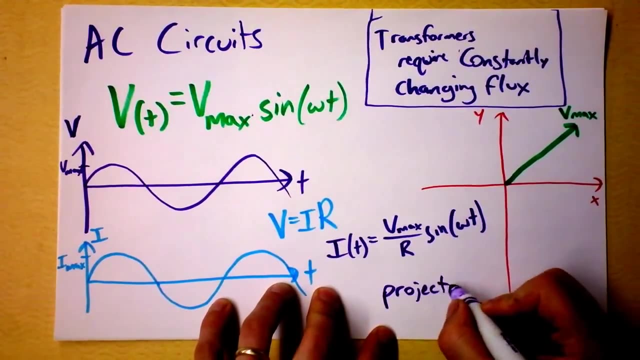 And the vector is continuously spinning around the origin. That's the definition of a phasor. And this phasor, I'm going to say, is v max long, That's how long it is. And I want to say that the projection of phasor on y-axis is instantaneous value. 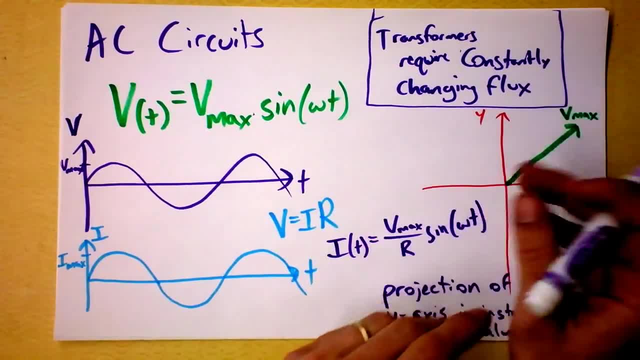 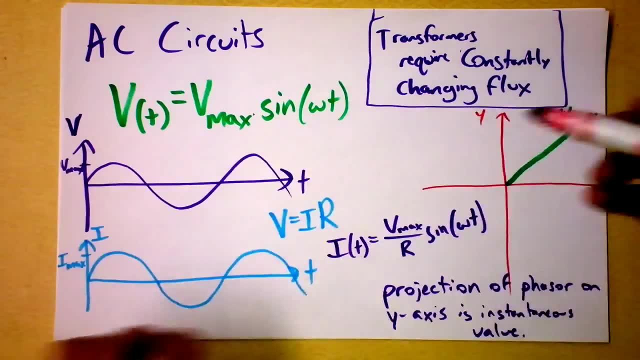 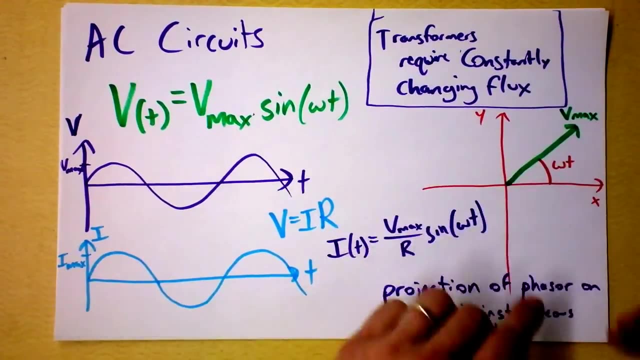 It helps to look at simulations of these at this point, because I'm not going to be able to rotate that, That vector around there, But if you know that that sucker is rotating and I guess we need to label some of these angles. this angle is going to be omega times t, Because, well, that's what's. 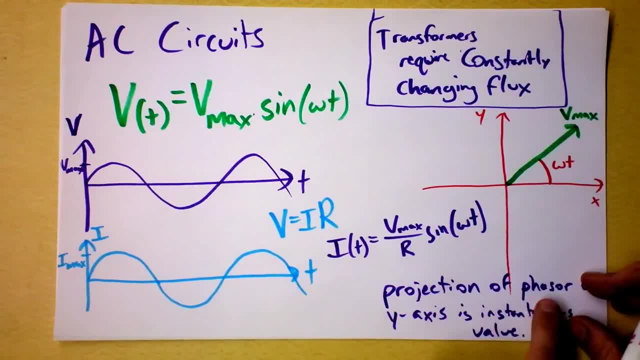 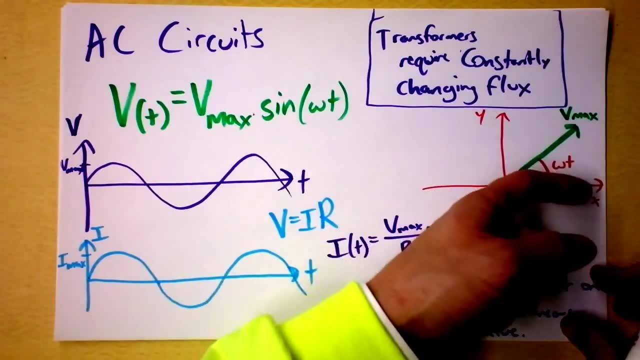 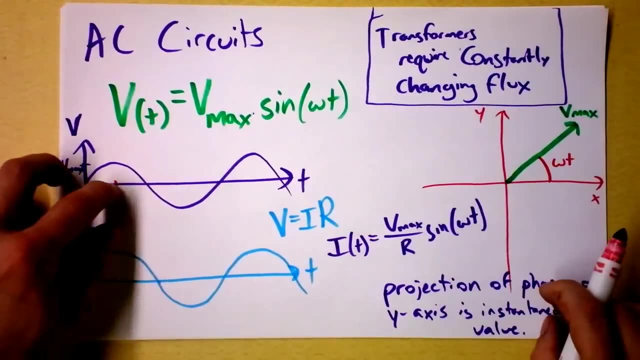 happening here. We initially have a y component, a y projection of zero, And it goes to a y projection of v max. And it takes the time, the time that it takes to do one quarter of a revolution gets us up to right here, Because that's a quarter wave, right. And then, as it goes around, 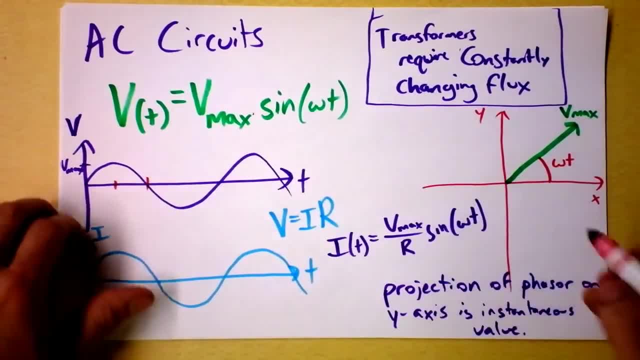 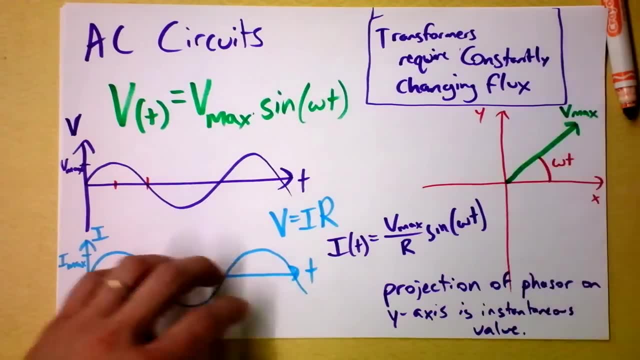 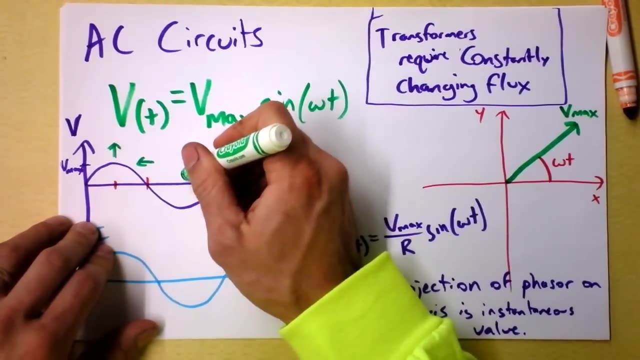 it goes back to zero again. Yeah, that's right here, This. maybe I can draw you some lines that correspond to various points, When, yeah, yeah, I can do that. I can show you the phasor in its orientation. So here the phasor is directly up, Here the phasor is directly to the left, Here the 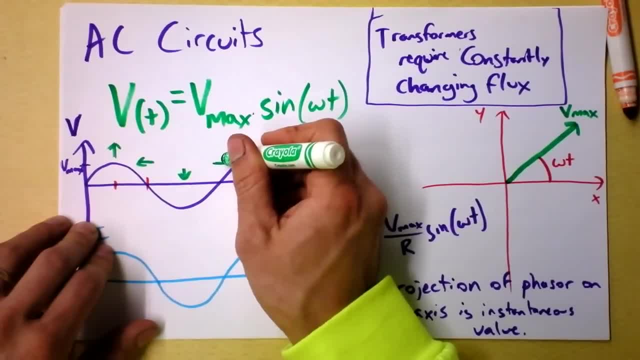 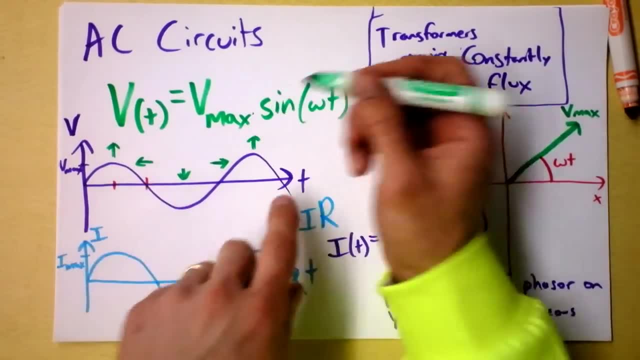 phasor is directly down Here. the phasor is directly to the right Now. it doesn't matter whether it's left or right At this point, But whether it's up or down tells us whether we have a positive or a negative. 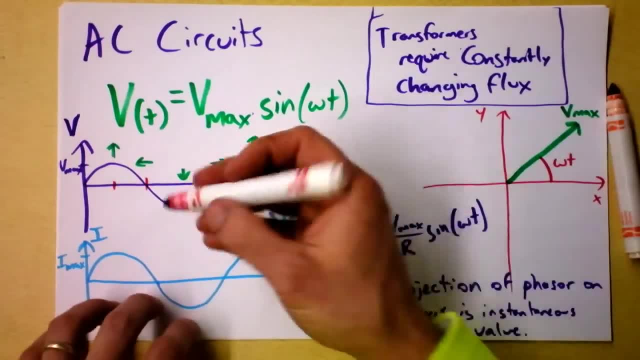 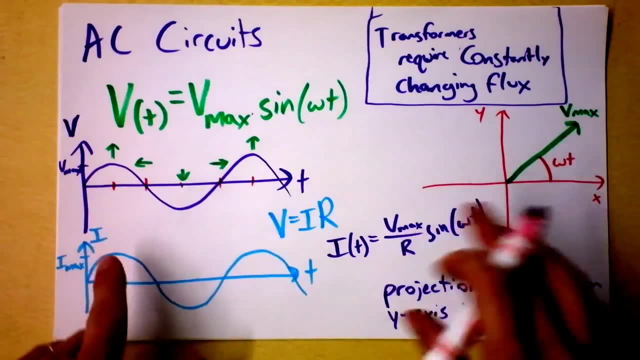 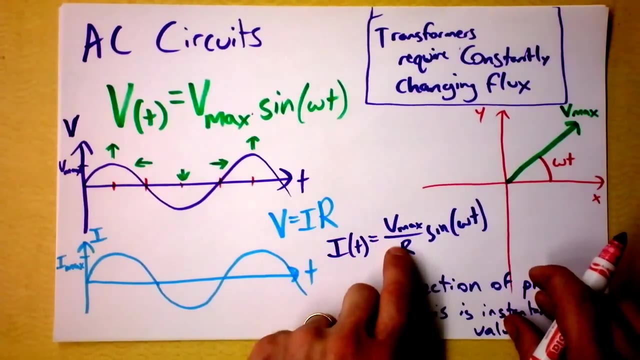 projection of the vector. So we can put little tick marks all along here and sort of acknowledge that it's these points that we're getting maximum or zero values for our voltage. But remember I said that the current is doing the same thing, But of course it's v max divided by r. So I 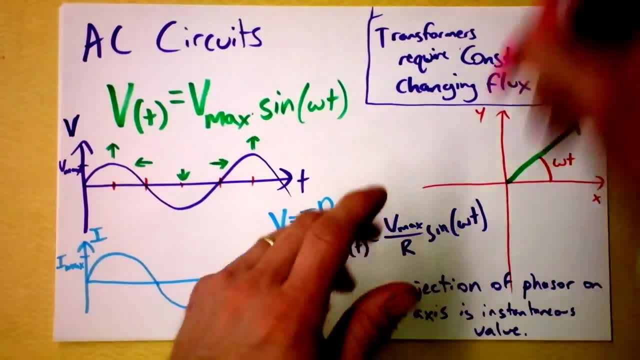 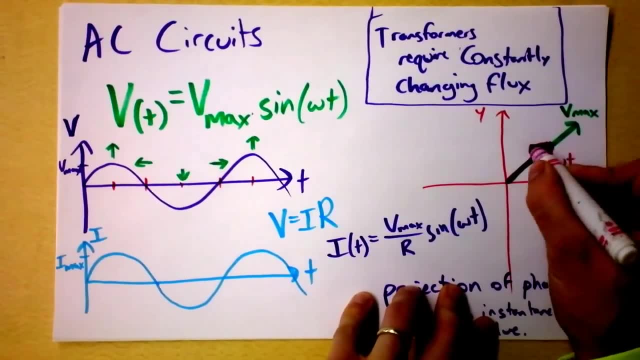 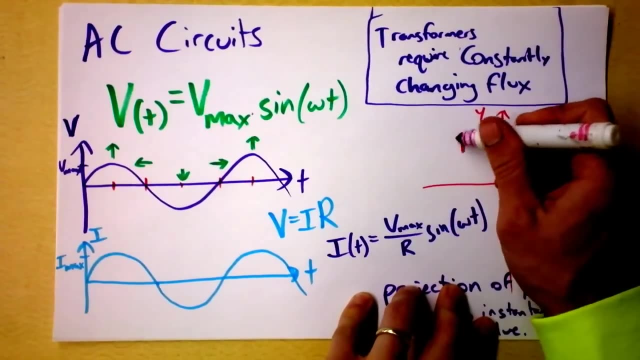 don't know what r is, But I can draw you a similar phasor, maybe right next to that other phasor- It actually should be right on top of it- And this phasor's length right here is v max over r, And v max over r defines I max. 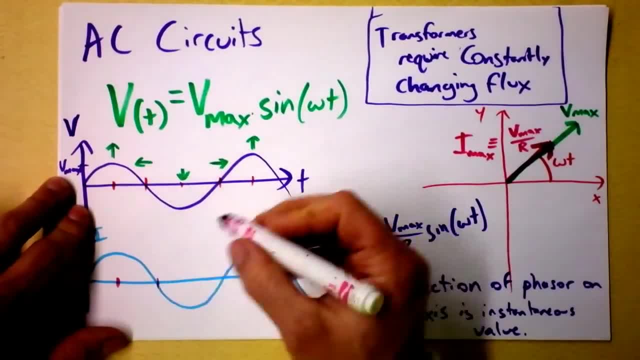 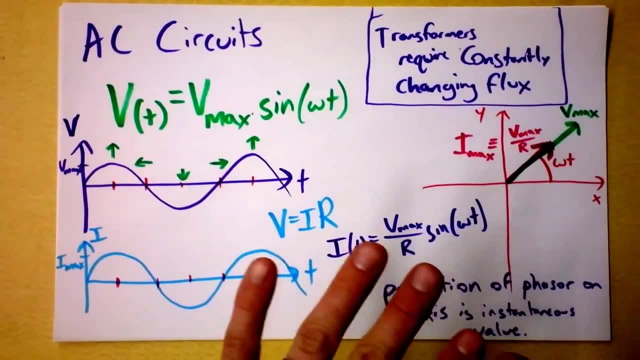 So, in a similar way, at each of these tick mark times, I can say that we have the same orientation for the I max vector. What that means is when there is a maximum current, there is a maximum voltage, and vice versa, Because those guys- oh, you got language for this. 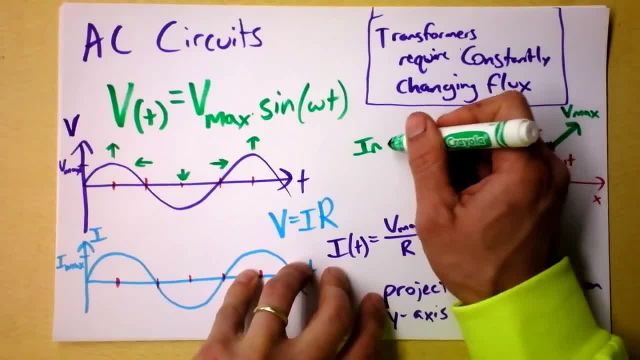 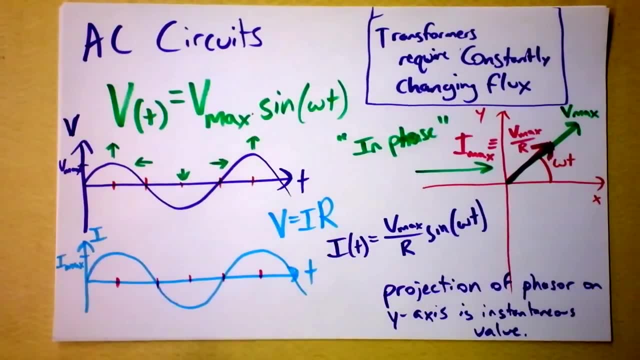 These guys are said to be in phase. They're said to be in phase because the phasers line up with each other, So that means if one changes, the other changes and they have the same time dependence, Uh-huh, uh-huh. 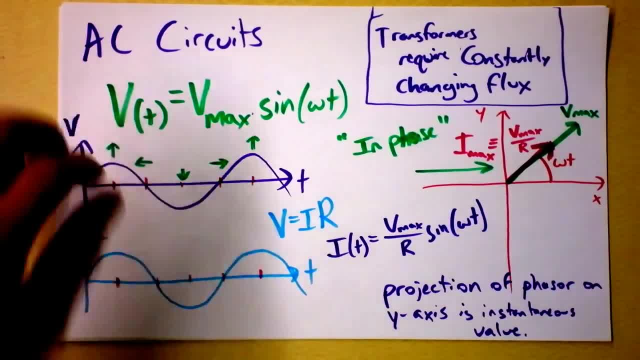 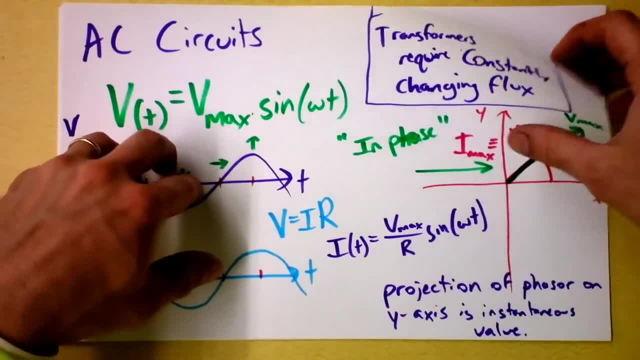 Now let's think about the definition of. well, I don't like the changing all the time. I would like a value to describe what it actually is, And I'm going to use a value called average. The problem is: what's the average of this graph? 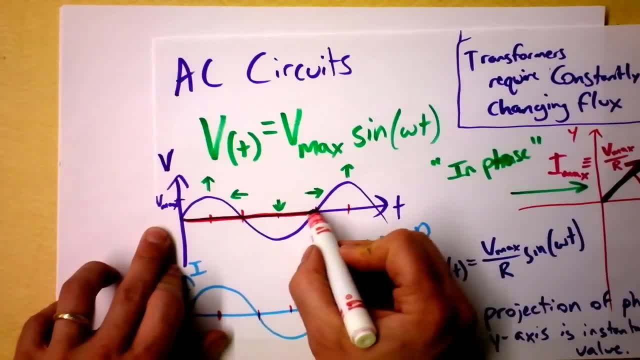 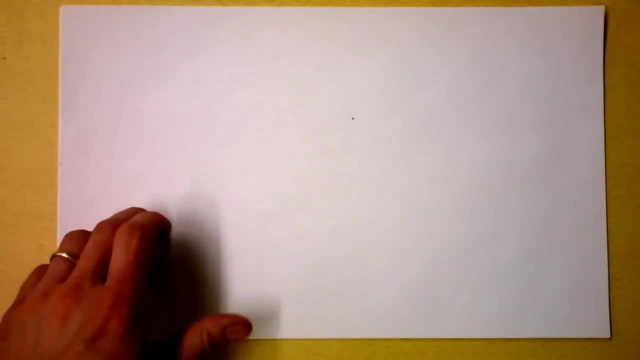 Well, let's see, It spends half its time up and half its time down. The average of that graph over one full rotation: Nothing. And the average of that over an extra rotation: Nothing. So the average isn't going to help us at all. 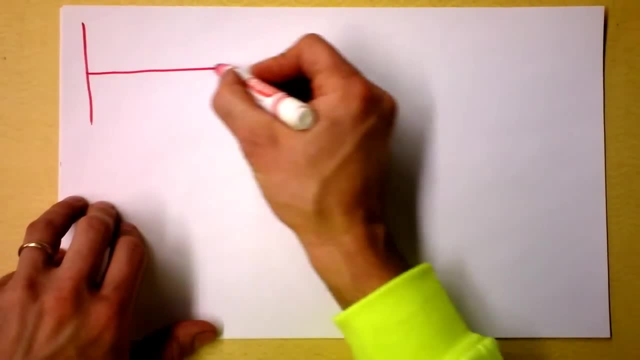 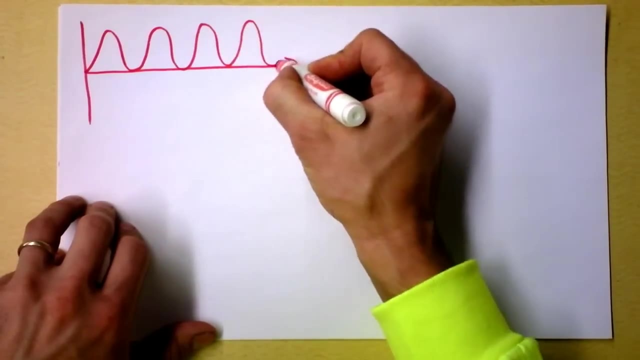 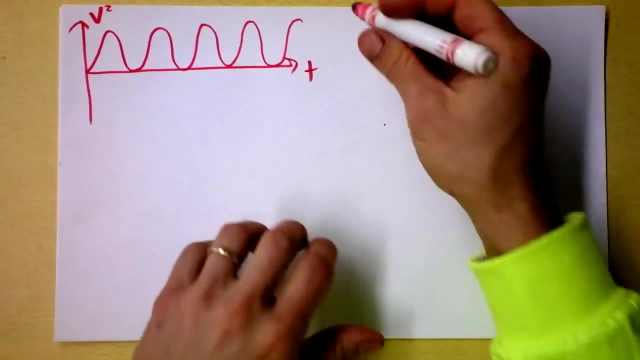 But what if we square it? Do you know what the square of the sine function looks like? The square of the sine function is like: So that's time and that's voltage, for instance, But it's voltage squared, And so voltage squared is. 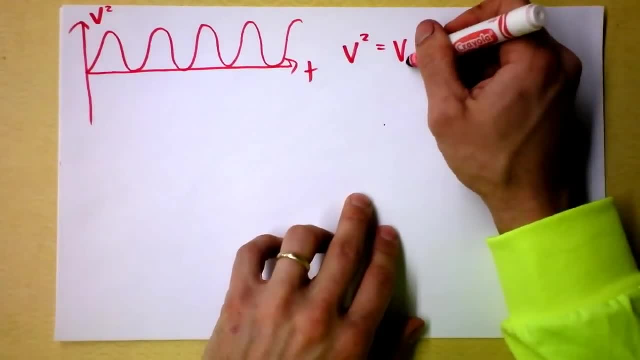 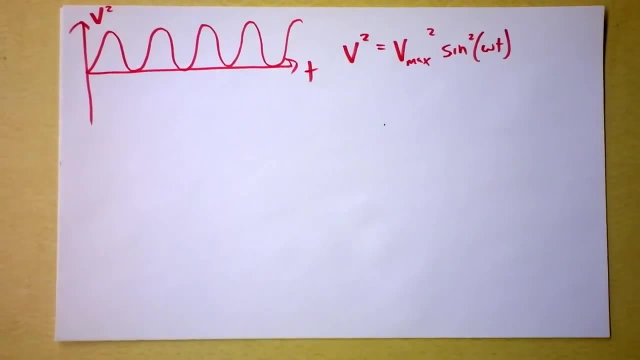 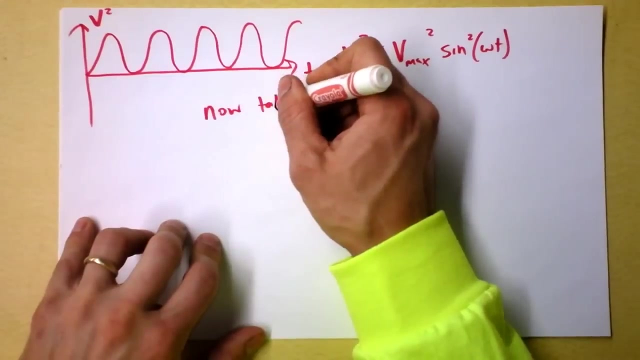 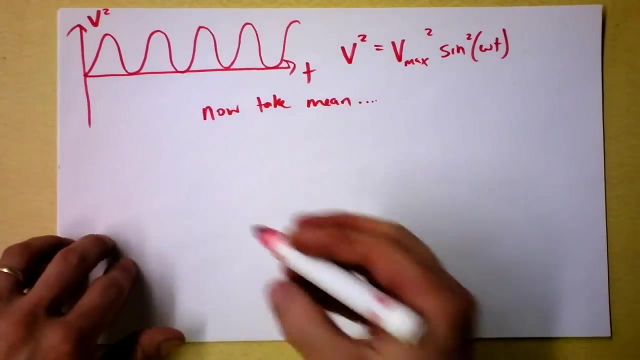 Let's look at that. It would be v max squared times sine squared of omega times t. So v squared still depends on time. But what if I take the average of that, Now take mean. And if I take the mean of that, sucker right there. 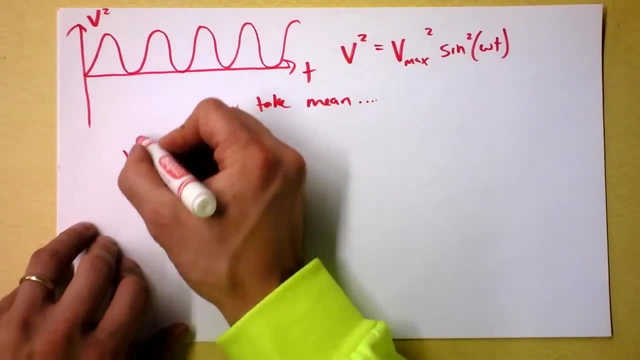 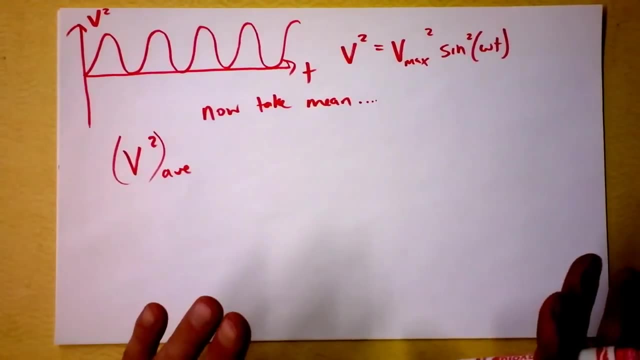 I'm going to say v, squared, averaged. No, I can't average and then square, because then it just gets zero. But if I take the square and then average it, then I'm looking for this value right here. Where do you think that is? 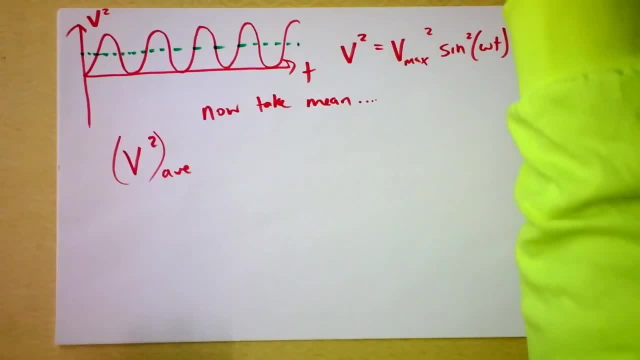 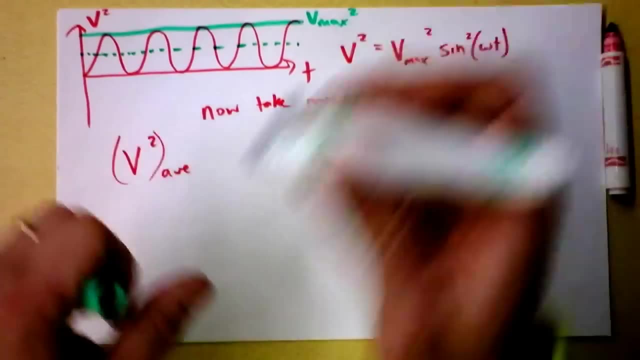 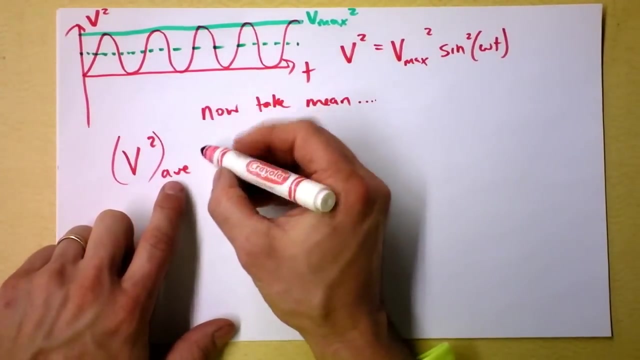 You see this value up at the top. this top value is what That top value is, simply v max squared, right? That's what it means. v squared max is v max squared, so that's fine, But v squared averaged is just half that big. 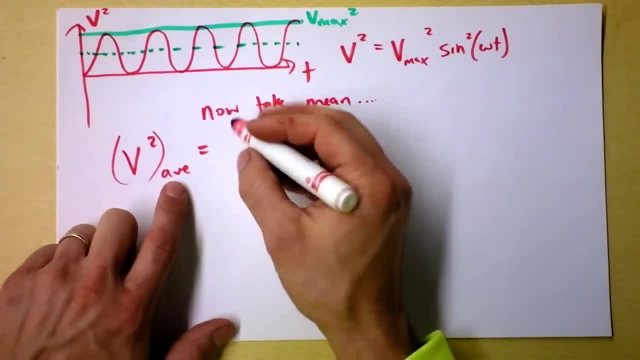 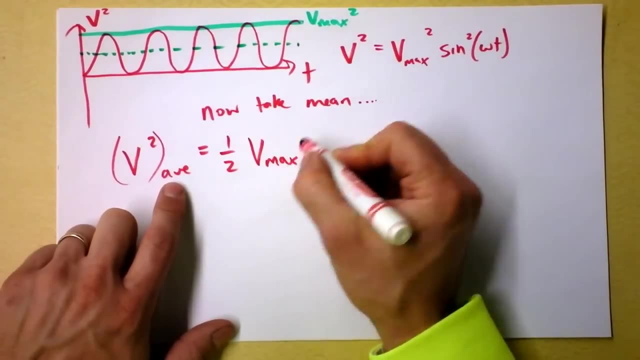 Look at it, Isn't it half that big? Of course it's half that big. It's symmetric around the halfway point. So this is one half. Now, careful, I'm going to write one half v max squared. Okay, All right. now here's my next plan. 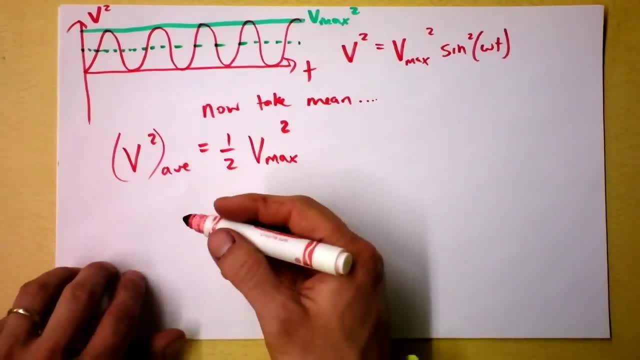 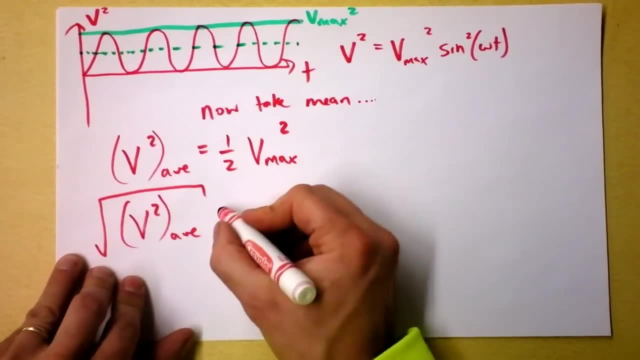 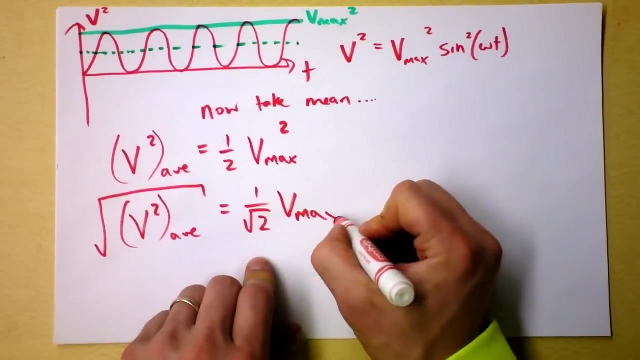 My next plan is to take the square root of this business right here. So I'm going to say v squared, averaged, and then screwed is well the screwed of that business right there. So this is one over screwed two times v max. Oh, that's a lovely conclusion. 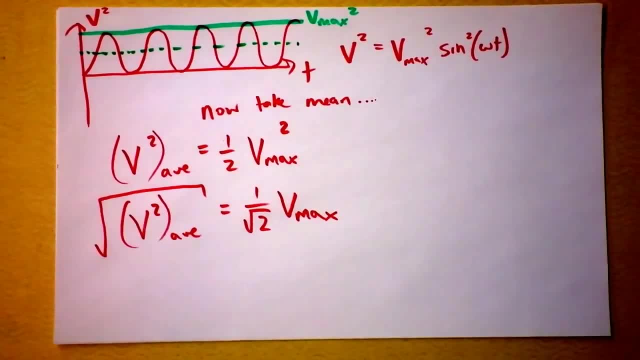 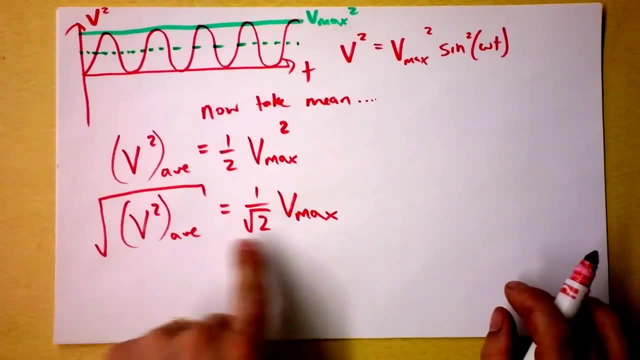 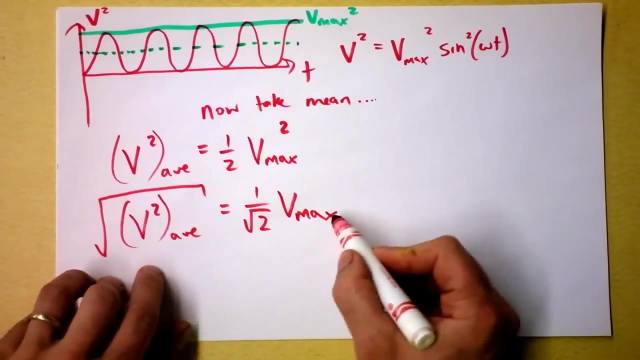 Wow, It turns out that every- Excuse me, Every- Every relationship where you've got a sign has the same functionality right here. If you square it and then average it and then screwed it, you will get one over root two of the maximum value of that function. 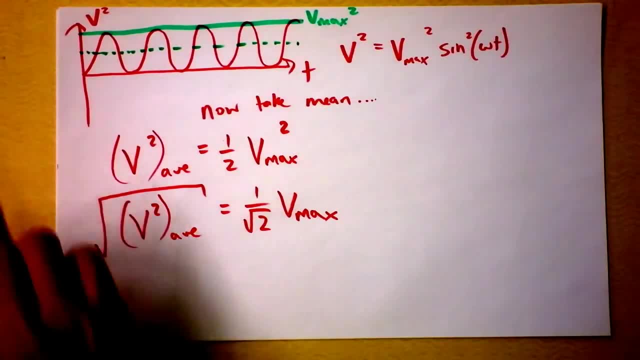 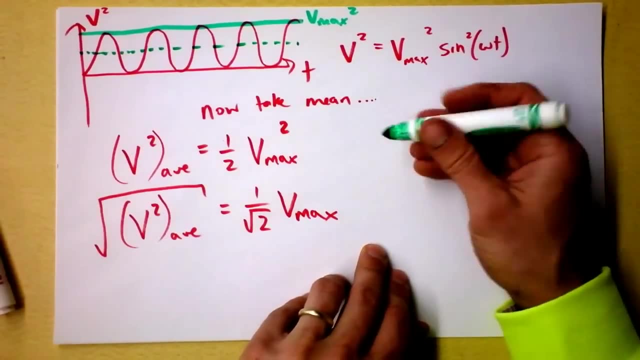 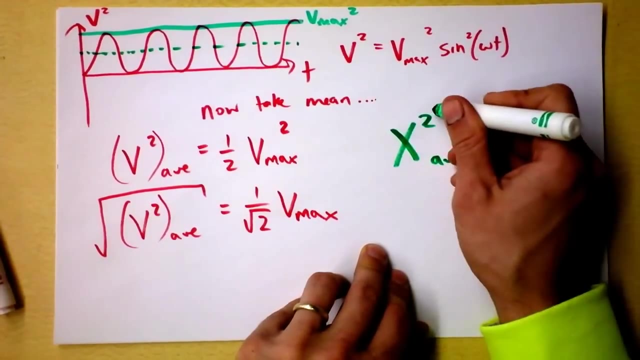 That's really lovely. So I can say, in a general sense, this will work for current and it will work for well, frankly, anything that is changing sinusoidally or cosinusoidally. I take any variable and I square it And I average the square and I screwed it. 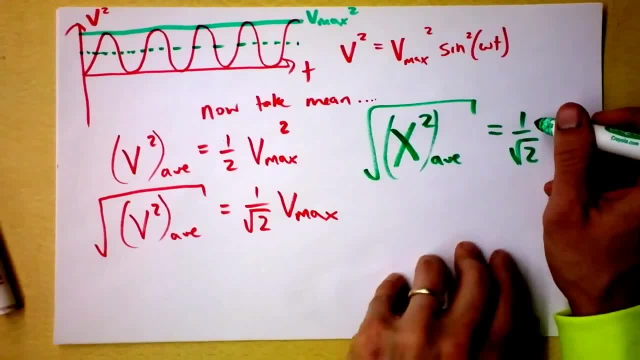 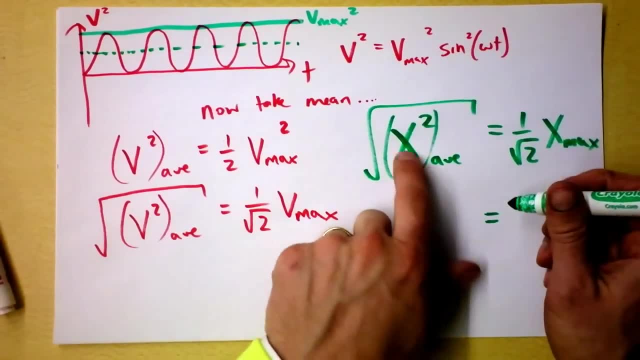 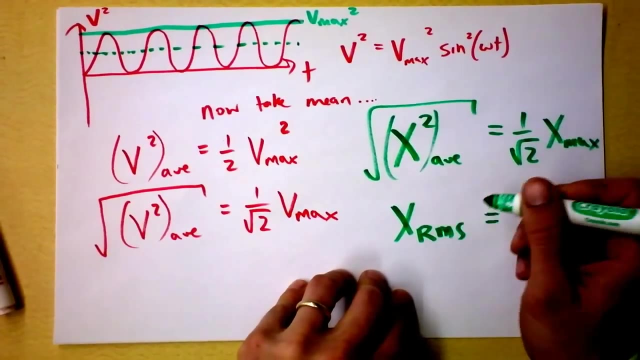 And this is one over root, two times the maximum value of that variable. And this thing right here, this squaring and then meaning and screweding, is called the RMS value. It stands for root, mean squared, because I'm taking the root and I'm taking the mean and I'm squaring it. 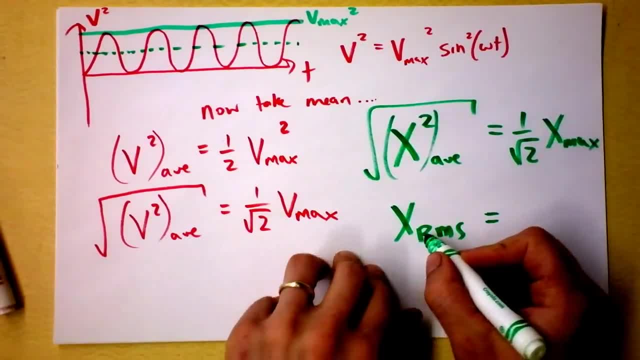 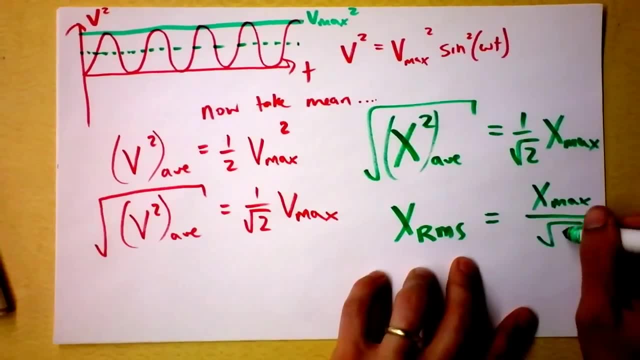 Not in that order, though. I'm squaring mean rooting it, But it's called root mean square, So you have to get used to that. And this is just whatever. the maximum value of that sucker is divided by root two. So let's say a couple of things and then I'll make some shout outs to you. 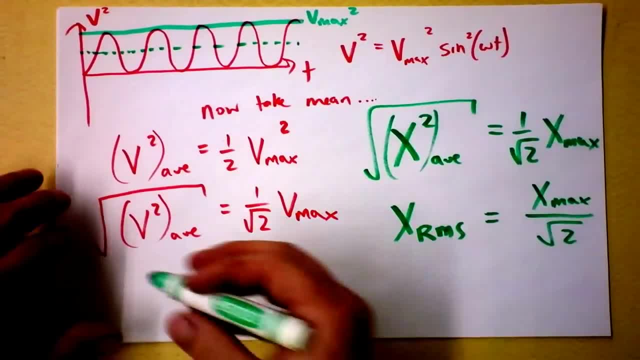 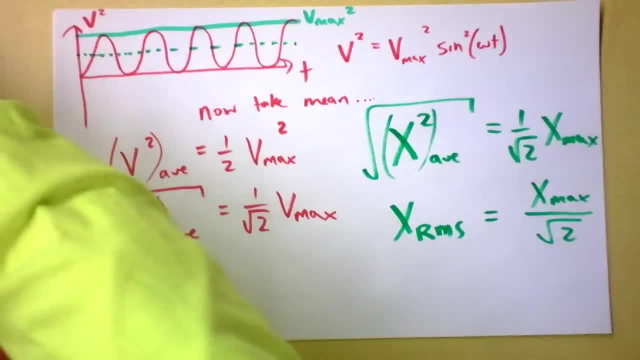 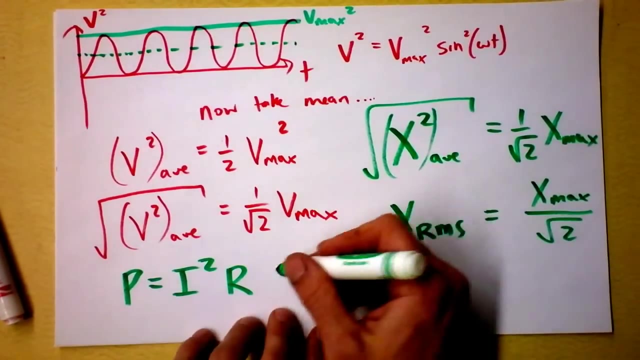 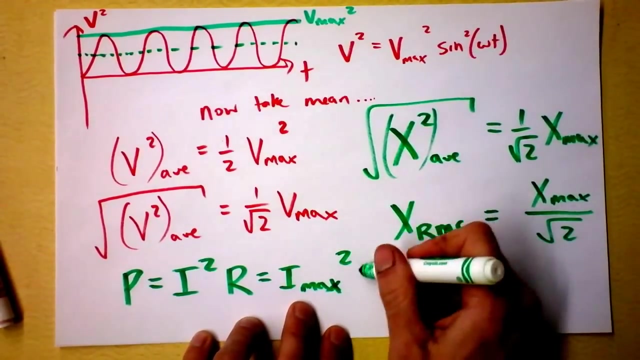 There's Well, there's power, right, And you know that power in a resistor like my hot plate, Power is I square times R, And if power is I squared times R, then it's simply going to be I max square times R. 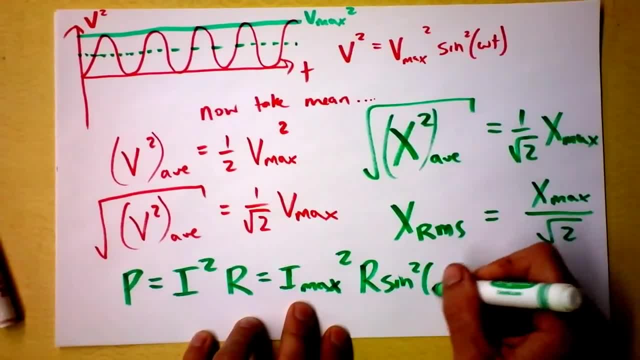 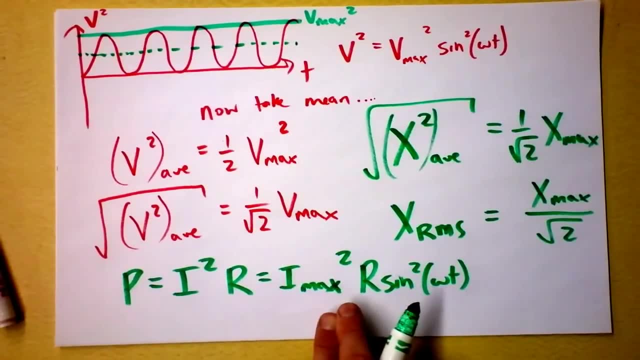 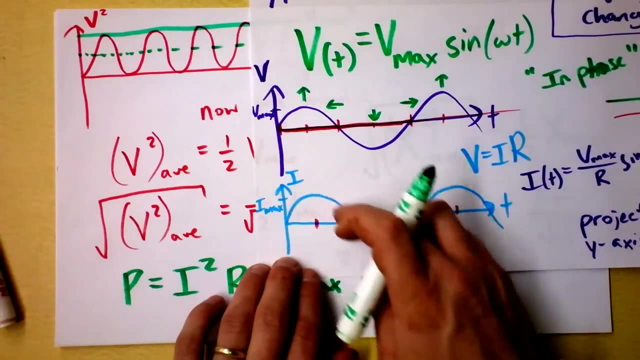 Oh, and then there's this sine square of omega t, But that, You see, this works instantaneously. This is the power at any instant, But the voltage and the current are changing sinusoidally. So at these instances, right here, 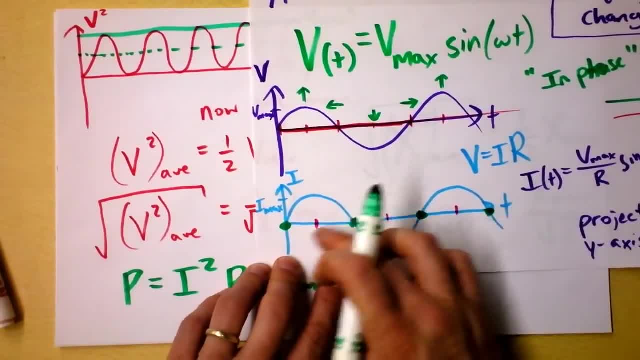 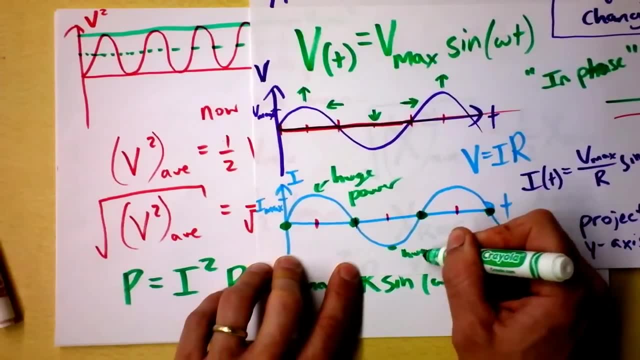 the power delivered by the circuit to my resistor is actually zero, And here this is huge power. And this is also huge power. It doesn't matter that the current is going the other direction In a resistor: it's going to heat up either way. 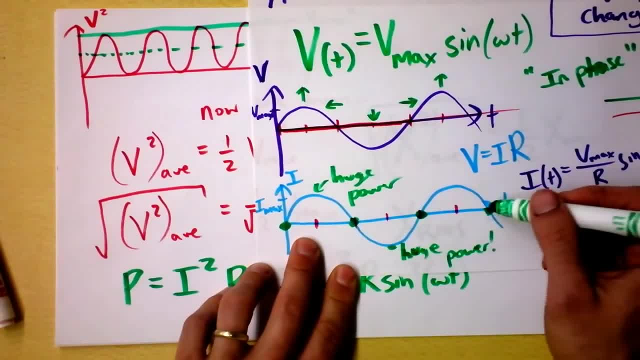 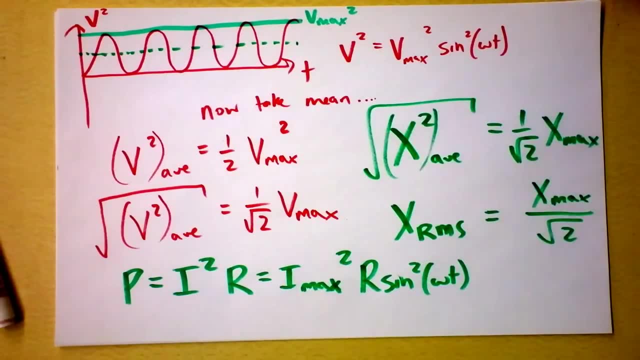 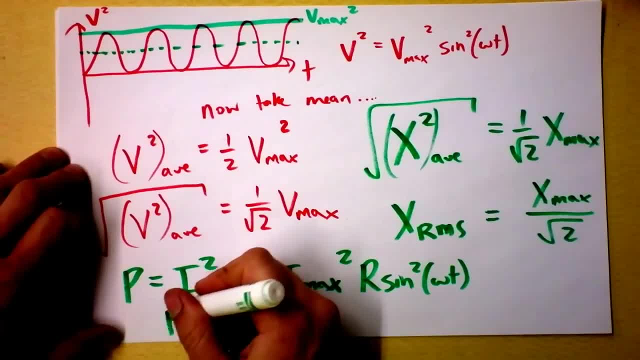 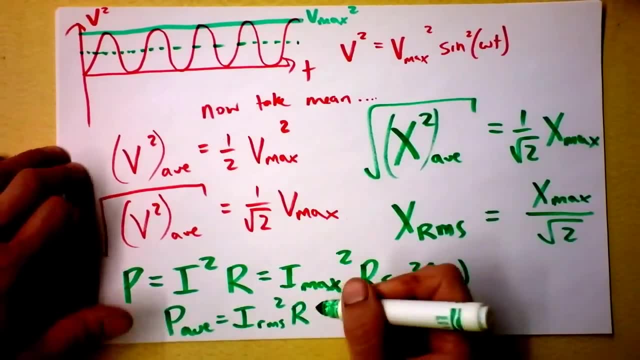 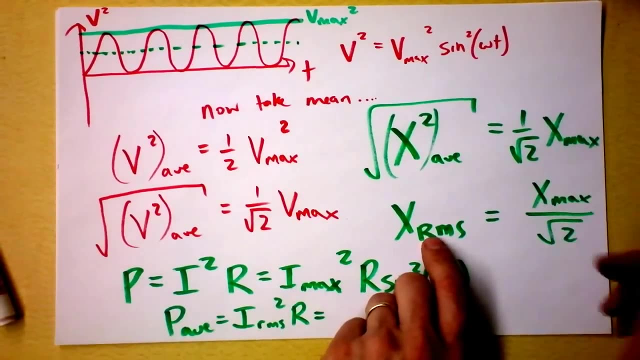 But I can tell you another equation like power: average equals current RMS Square times R, And So that means: Wait a second. The average power. Wait, if I take, I RMS this thing right here and I square it, I'm going to get. 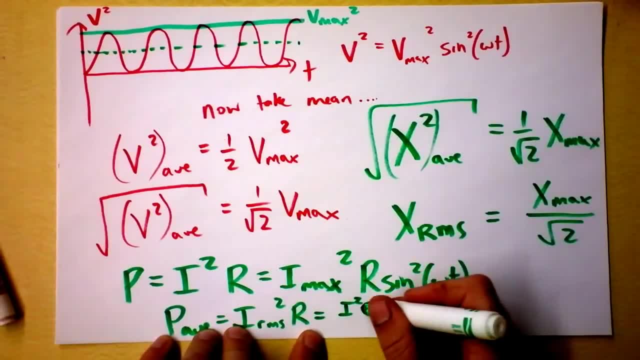 I Square. Wait a second. That's I max square times R divided by 2.. Interesting, All right, And this is true at any time. This doesn't have any time dependence, because I'm looking for average. The beautiful thing is. 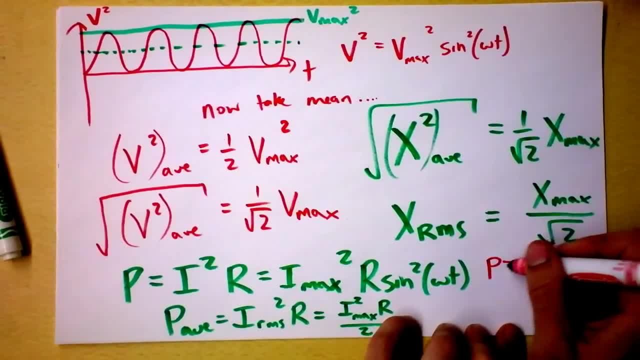 we've had all this complication and we get back all of our standard equations. Power is IV. As long as I use RMS, RMS, I'm still good. I can find the average power And I get power. is I square times R? 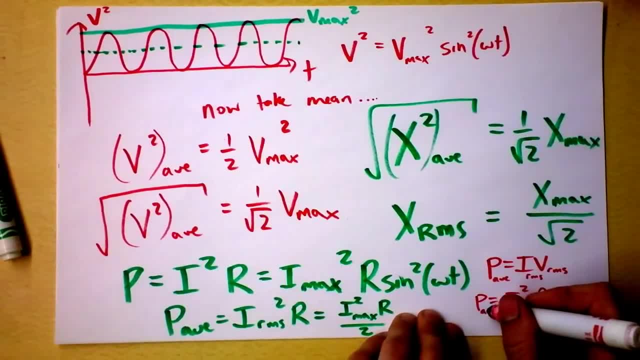 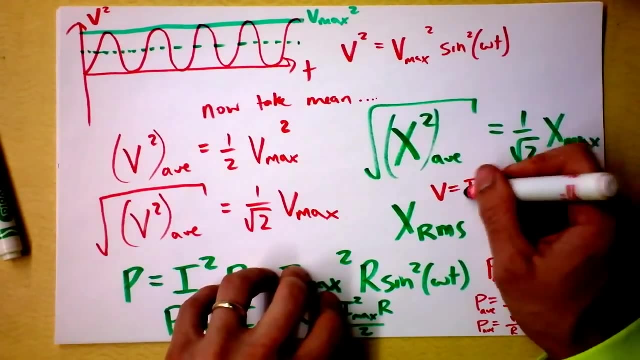 if I use RMS current, and then I will get average power. And we can also say that power is V square over R. If you use RMS voltage, then you'll get average power. Yay, Everything we knew already. Oh, and also V is IR. 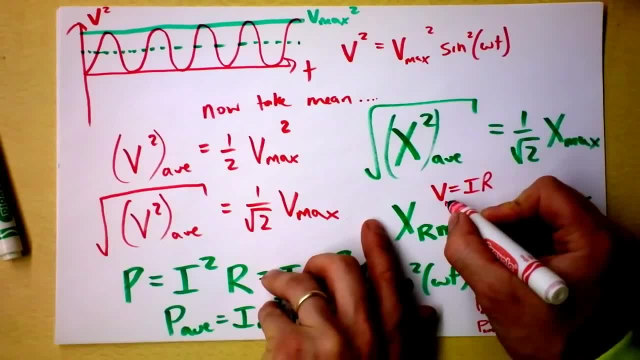 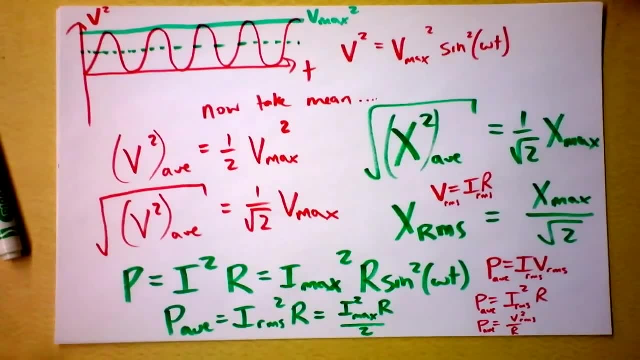 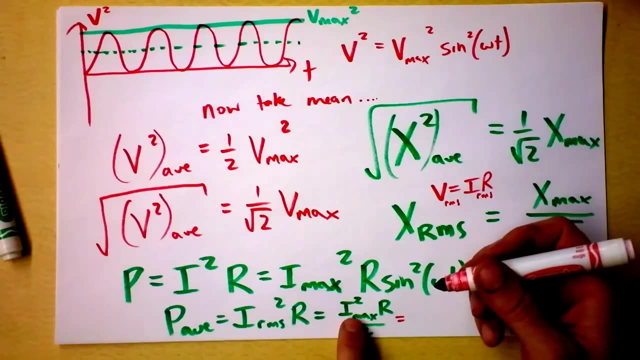 It's true that this is true instantaneously. but also the RMS voltage is the RMS current times, the resistance, RMS times, the resistance of our resistor. Yay, We got everything back. Now the only Oh, shoot This right here. average power. 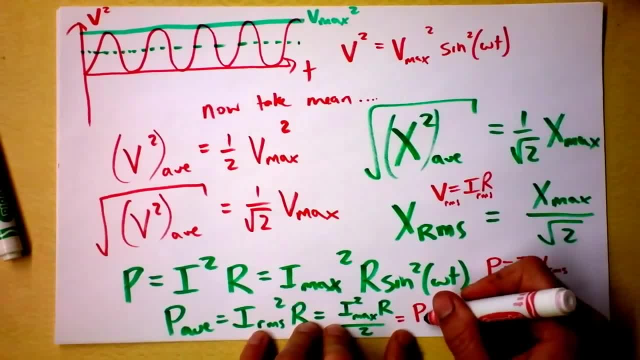 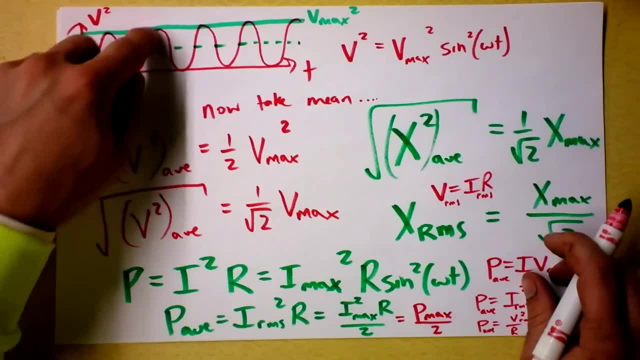 this right here I square max times. R is maximum power, So the maximum power divided by 2 is the average power, because power depends on the square of the current function, Or, depending on how you look at it, I guess it depends on the square. 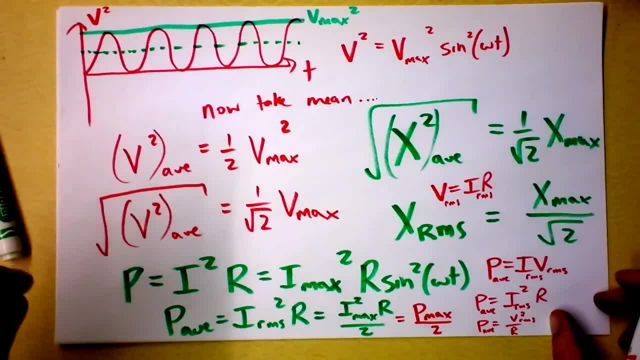 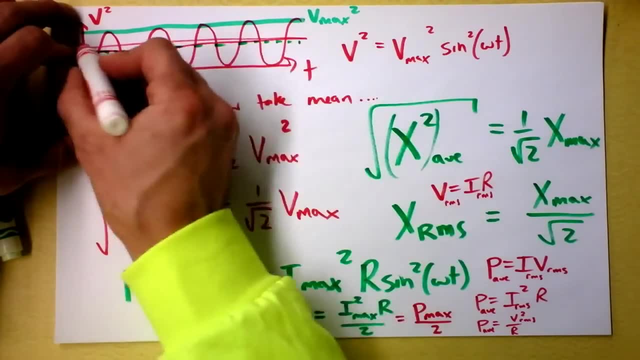 of the voltage function. So you've sometimes got zero power and you've sometimes got maximum power, but your average power is right smack in the middle of the average and the maximum, And that makes sense, I think. So let's look at just one example. 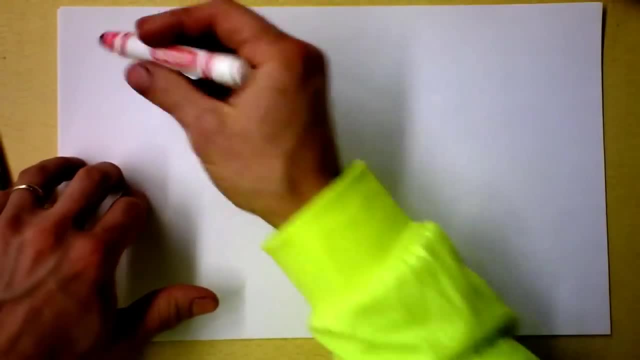 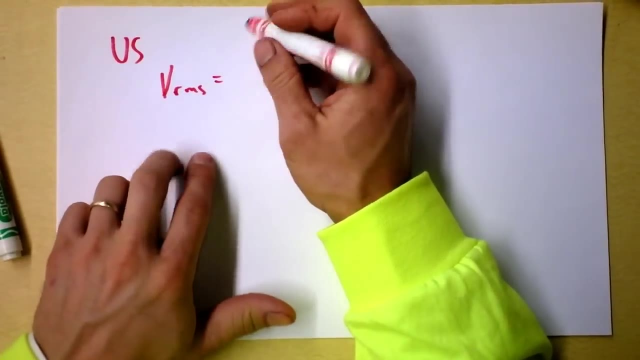 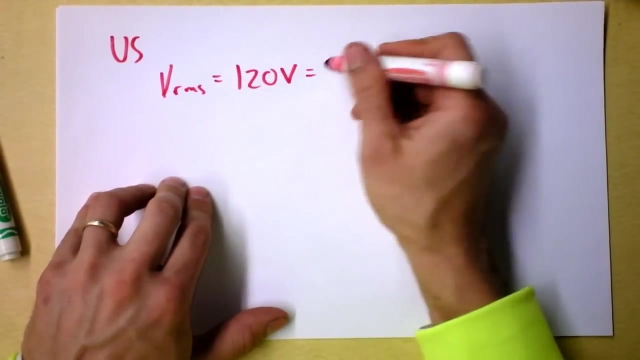 of this beautiful equation here, the RMS voltage. In fact US says that V RMS is. Oh, what do they say? They say the RMS voltage is 120 volts from my electrical supplier And I know that the RMS voltage is the maximum voltage. 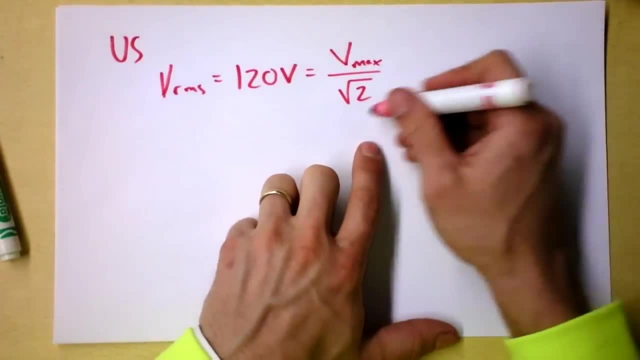 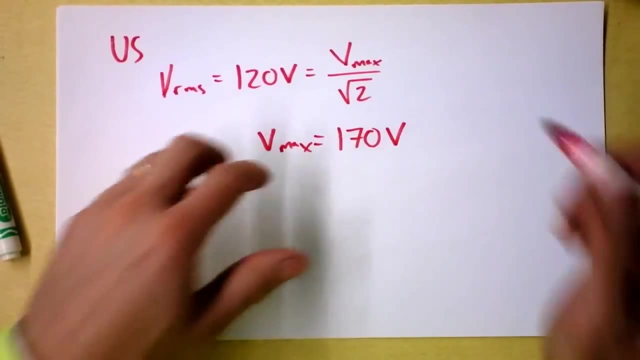 divided by the scroot of 2.. So I can find that the maximum voltage is: Oh, what do you get? 170 volts or so, Whoa, So they've been telling me it's 120 volts, but really it's 170.. 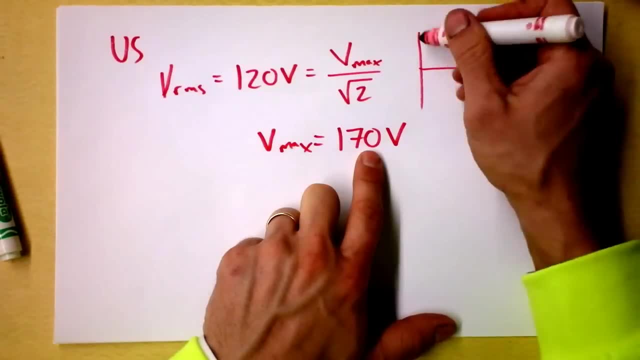 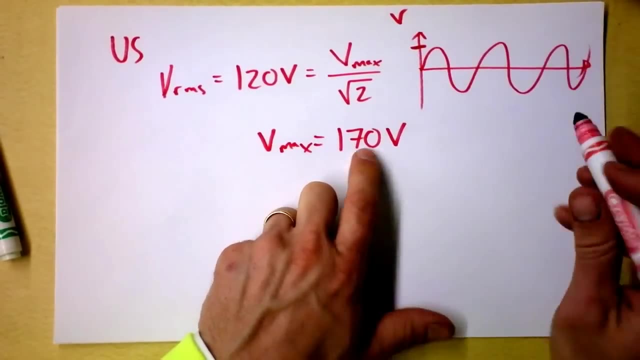 No, It's 170 some of the time. Here's voltage as a function of time and it's making this sine graph The maximum value. the maximum value is 170, but the RMS is 1 over root 2 of that. 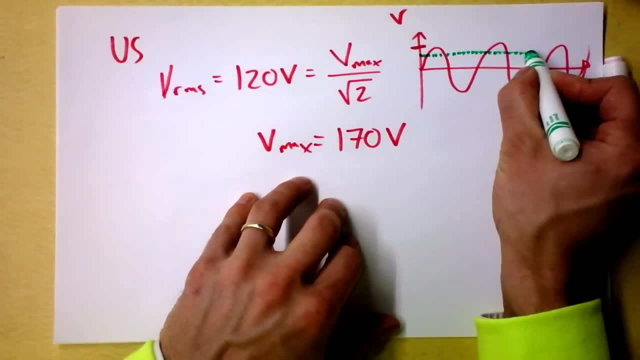 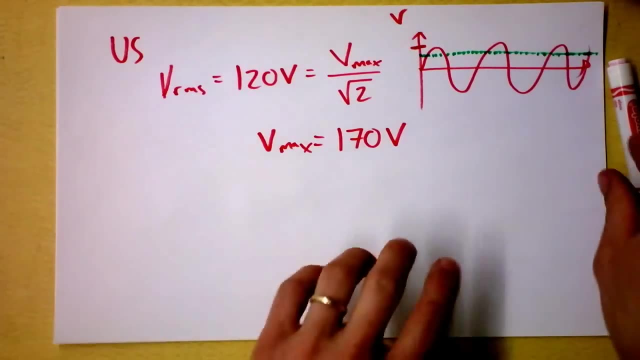 so the RMS is like right here. That's the RMS voltage And of course it's not the same thing as the average, because the average voltage is 0, but it's a way to indicate to us the amount of voltage that is there. 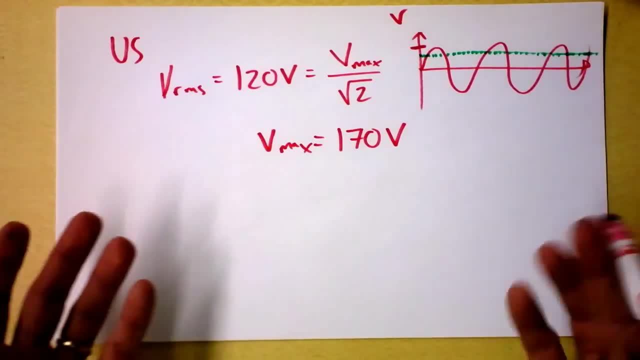 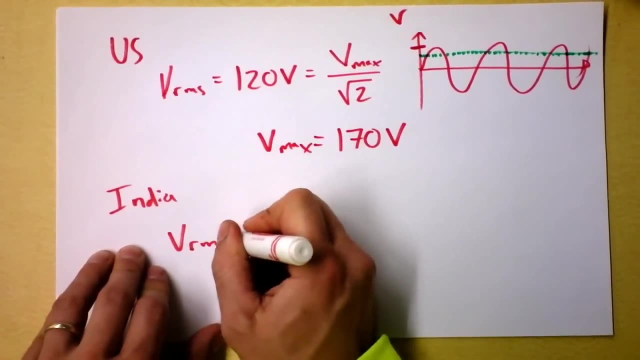 on a root-mean-squared kind of level. I don't know any better way to say it. And hello everybody in India. They tell me that your RMS voltage is. What do they say? I think they say that it's 220 volts. 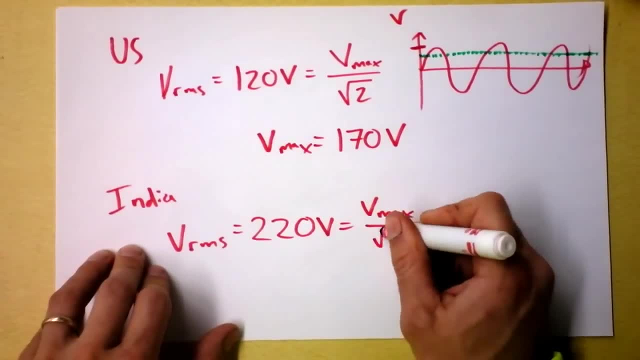 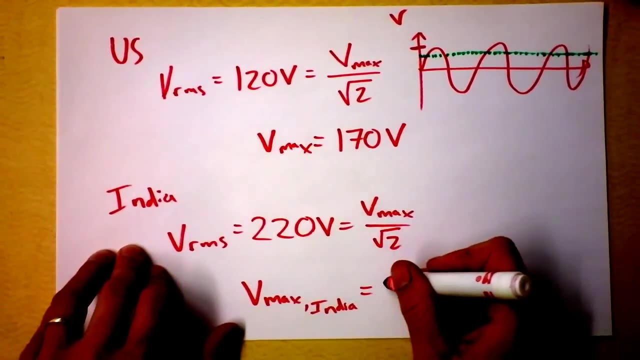 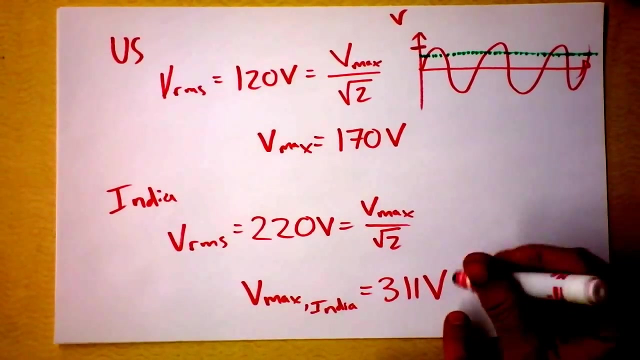 and that's your maximum voltage divided by the scroot of 2.. So the Vmax in India is about 311 volts, Wow, Okay. So I think in Europe they'd find it to be 320 or 330 volts. 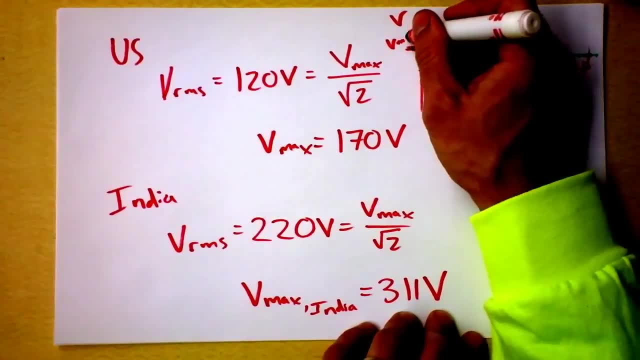 That's just the difference between the maximum value here and the RMS value that I've shown in green. Goodbye. 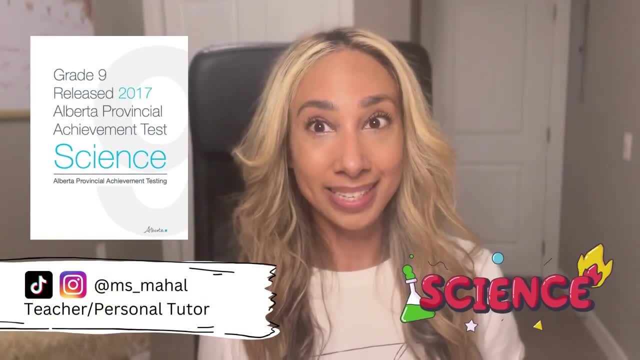 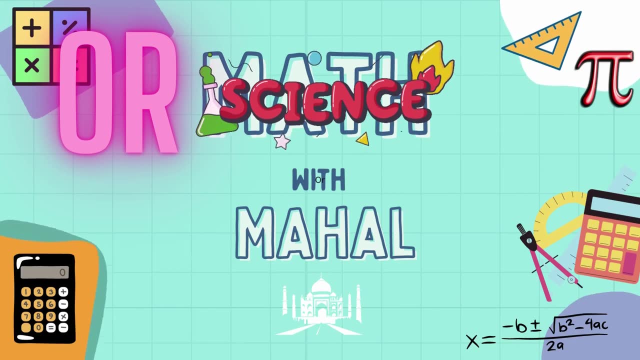 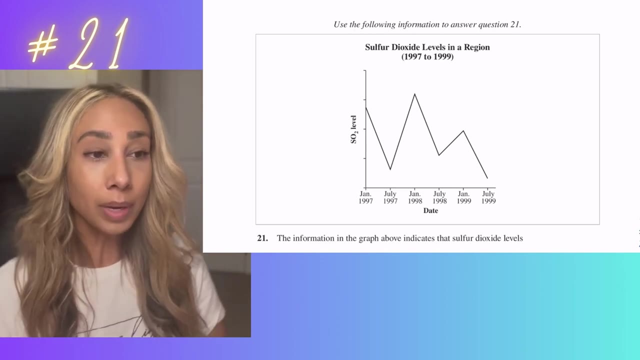 In this video I am going through the science 2017 PAT. This one, specifically, is looking at all the environmental chemistry questions. All right, so let's start here with number 21.. So we've got a graph and there's a couple of things we need to look at. So, before we even 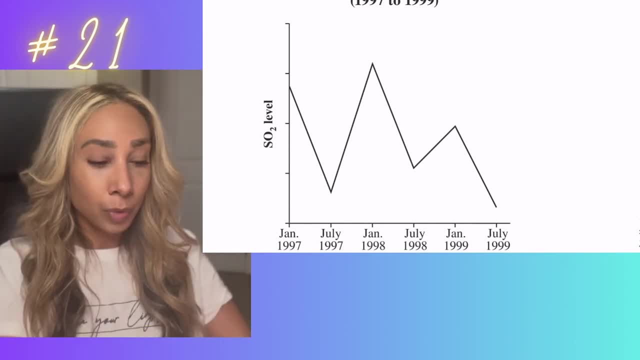 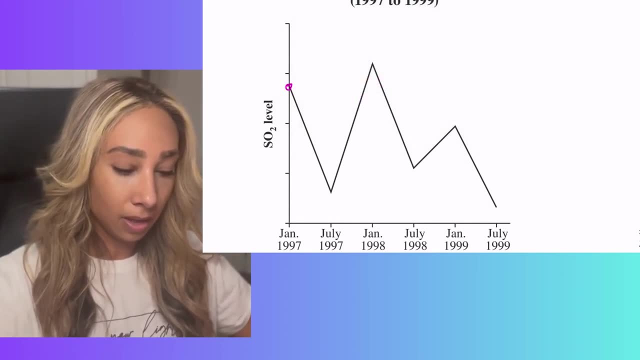 dive into the question. let's look at the graph and see what's happening. So, with our graph, there's a couple of things that I'm noticing right away. The first thing is that the levels of carbon dioxide- or, excuse me, of sulfur dioxide, SO2, start to increase around January. 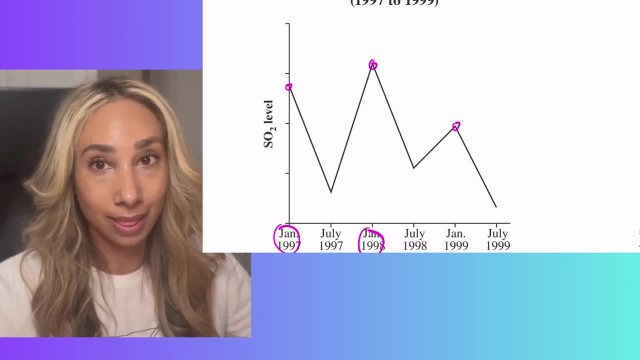 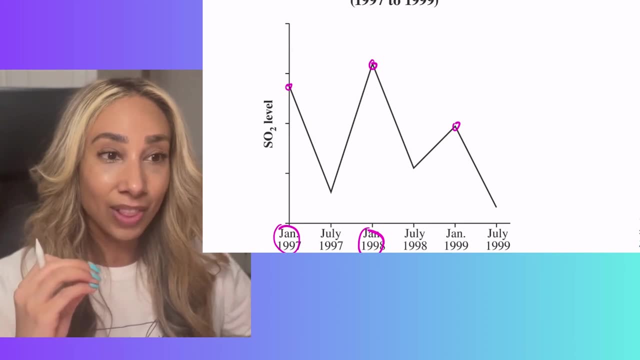 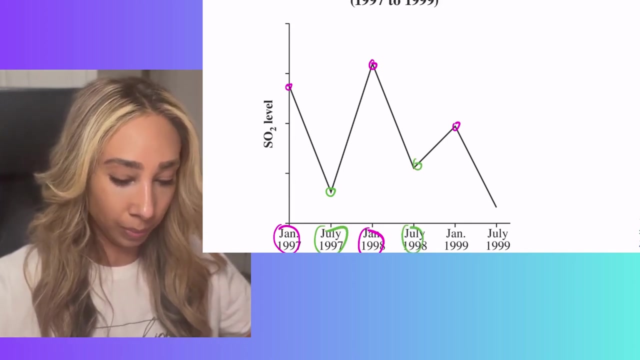 Okay, now take a look and see if there's anything else that you notice in this. The next part that I'm noticing is the levels of SO2 decrease in July. So we can see that they're decreasing here, decreasing here, and then they really decrease in July of 1999.. Overall, there 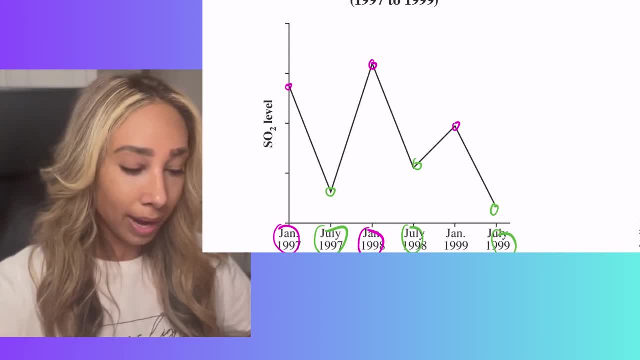 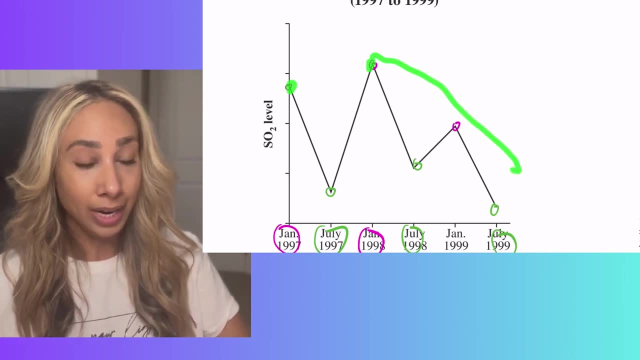 is like a general trend. If I look at the graph, I can see that the levels of carbon dioxide, the graph as a whole, where we kind of started high, had a little bit of a peak in 1990,- what is that? 1998, and then it went down overall. Okay, so there is this sort of like idea where it kind